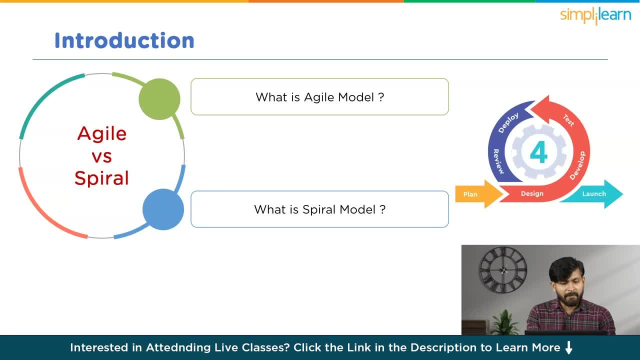 that incorporates elements from both waterfall and prototyping model. It addresses the challenges posed by large, complex projects, with focus on systematic risk analysis and management. Now, as you know guys, spiral and agile methodologies stand out to be the prominent software development approaches. Now, since we have got to know, a brief idea regarding 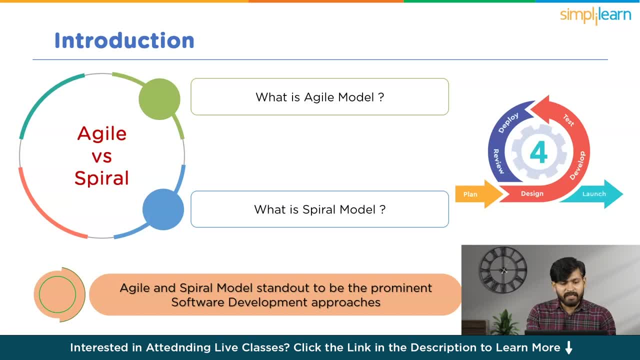 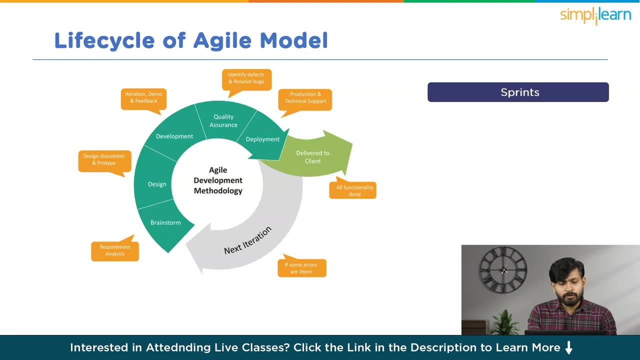 what is agile and what is spiral. let's move on to their lifecycle phase. Now, if I talk about the agile development lifecycle, guys, the agile development lifecycle is marked by short iterative cycles, known as sprints. These typically last for two to four weeks and involve planning. 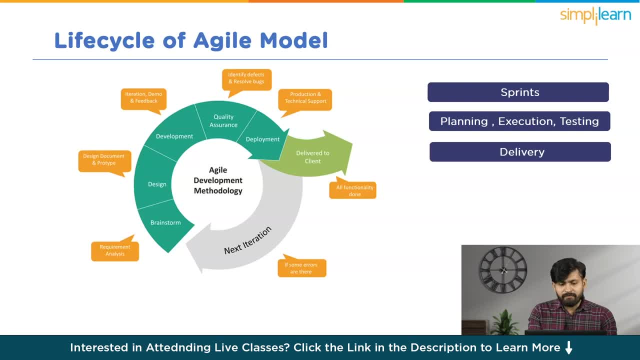 execution, testing and delivery. The iterative nature of agile promotes continuous improvement, as each sprint incorporates feedback from stakeholders. Popular agile frameworks include Scrum, Kanban and Extreme Programming. It provides specific methodologies for their effective implementation. Similarly, guys, let us discuss about the lifecycle of spiral model. 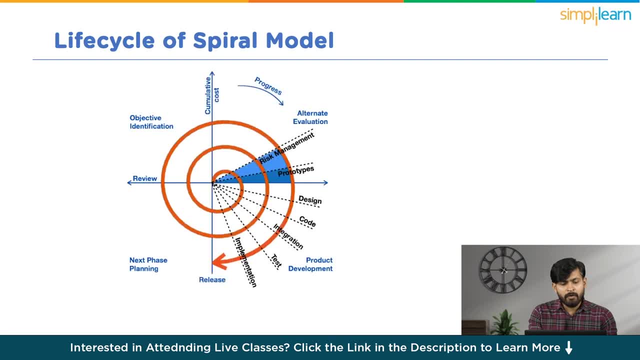 If I talk about the spiral lifecycle guys, the spiral model lifecycle consists of multiple iterations or spirals, each containing phases such as planning, risk analysis, engineering, testing and evaluation. These iterative approaches accommodate changes and enhancements as the project progresses. The model concludes when the software meets predefined objectives. 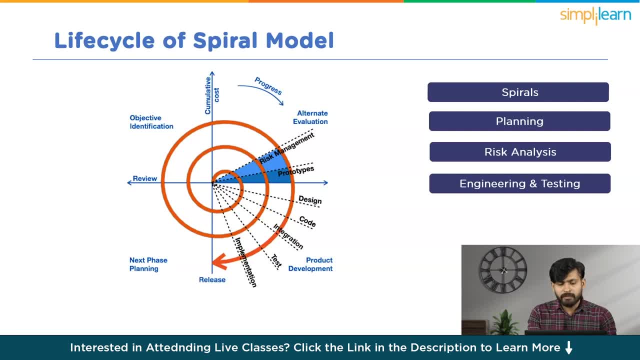 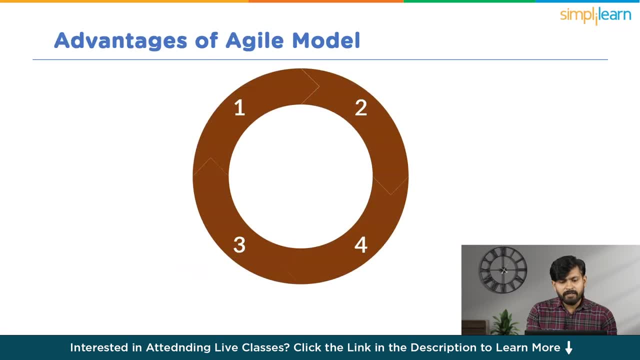 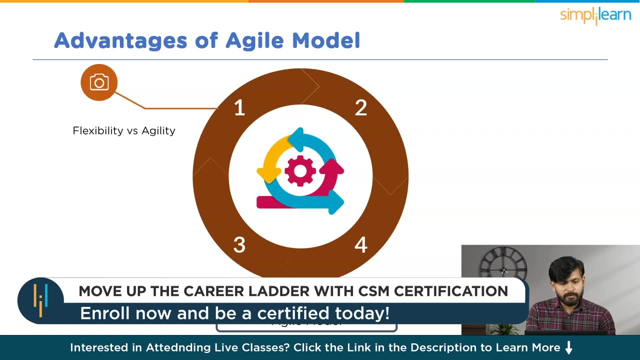 and satisfies stakeholders' requirements. Now let's move on to a discussion about the advantages of the agile model. If I talk about the advantages of agile, the first one that comes to my mind is flexibility and adaptability. If I talk about flexibility, guys, agile's iterative nature allows for. 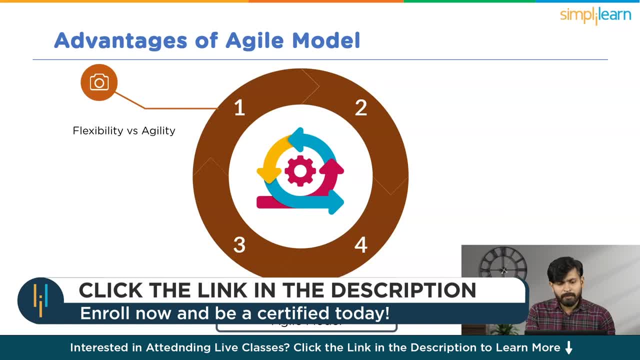 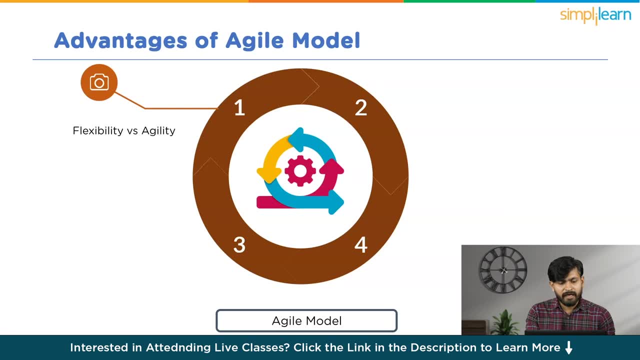 rapid adaptation to changing requirements. This adaptability is crucial in today's dynamic business environments, where client needs and market conditions can shift unexpectedly. The next one is customer satisfaction. The continuous involvement of customers and stakeholders ensures that the delivered products align closely with their expectations. Regular feedback loops. 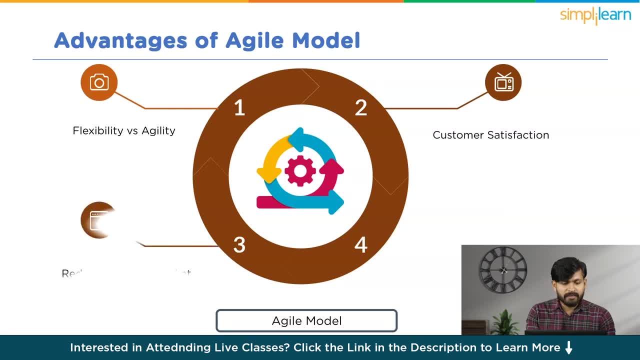 contribute to higher satisfaction rate. The third thing is reduced time to market. Incremental development and frequent releases in agile lead to a reduced time to market. This agility in delivery is particularly advantageous in industries where being first to market can be a competitive advantage. The next one is improved quality. Agile's emphasis on 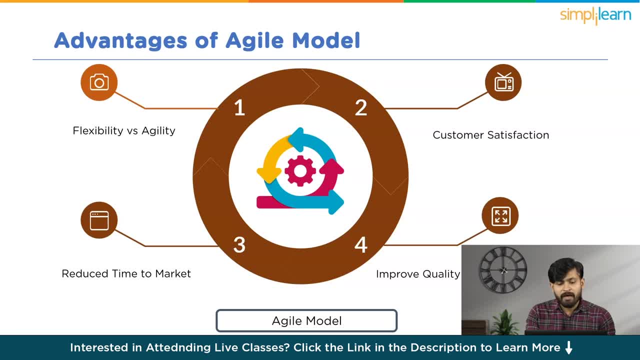 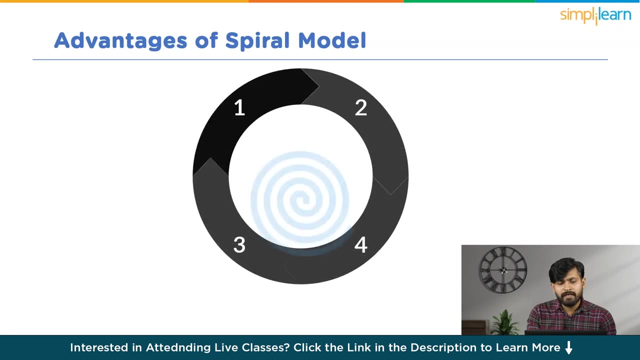 continuous testing and integration practices contribute to higher overall software quality. By addressing issues early in the development process, the final product is more reliable. Similarly, guys, if I discuss about the advantages of spiral model, the first one that comes up to my mind is risk management. The spiral model's unique strength lies in its approach. 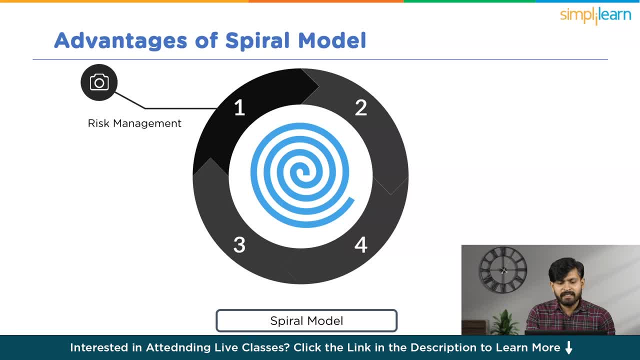 to risk management. By systematically identifying, analyzing and mitigating risk at each iteration, it offers a proactive strategy to handle uncertainties. Next one is flexibility and changes. Adaptability is a key feature of the spiral model. Changes and requirements can be seamlessly integrated. 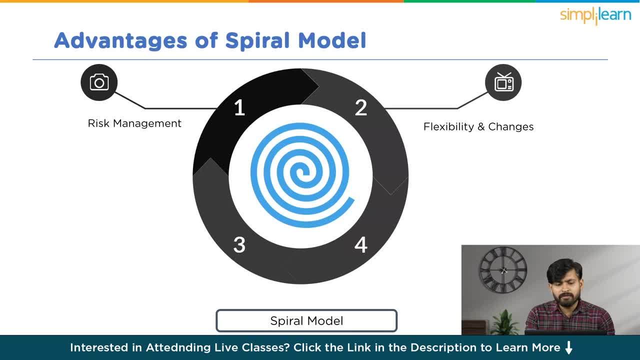 into subsequent spirals, ensuring the development process remains aligned with evolving project needs. The next one is it's highly customizable, Tailored for projects with dynamic or uncertain requirements. the spiral model is highly adaptable to different development scenarios. The high level of customizations makes it suitable for diverse project environments. 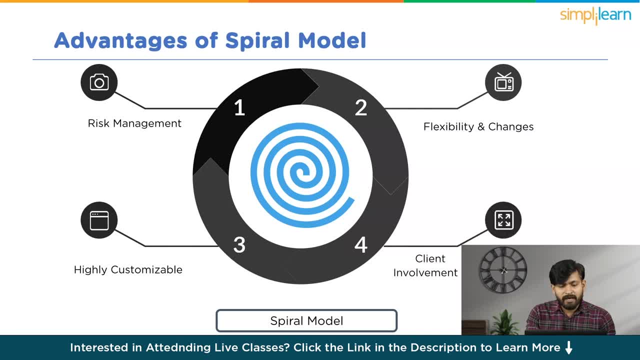 The fourth one is client involvement. Regular feedback from stakeholders ensures that the final product aligns with the user's expectations. The spiral model's iterative nature allows for continuous client involvement, fostering a collaborative development process. I hope so. you would have got a brief idea regarding the advantages of agile and spiral model. 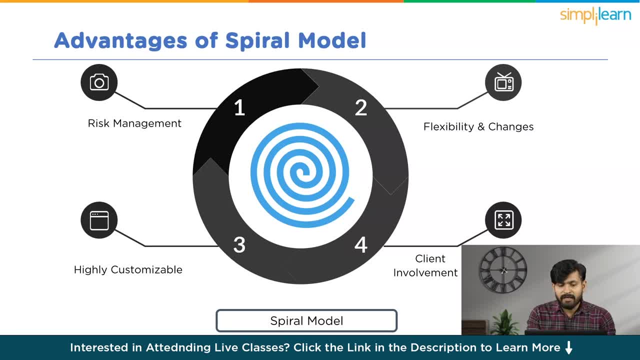 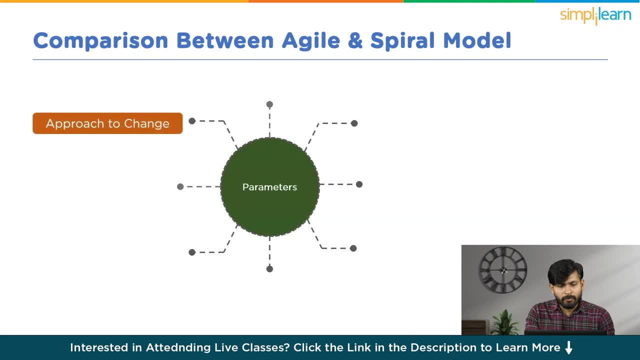 Now let us jump to the main part, that is, the comparison, and let us see how agile is different from spiral. So, guys, the first parameter that comes up to my mind is approach to change In agile model. if I talk about it, its approach to change is characterized by its flexibility. 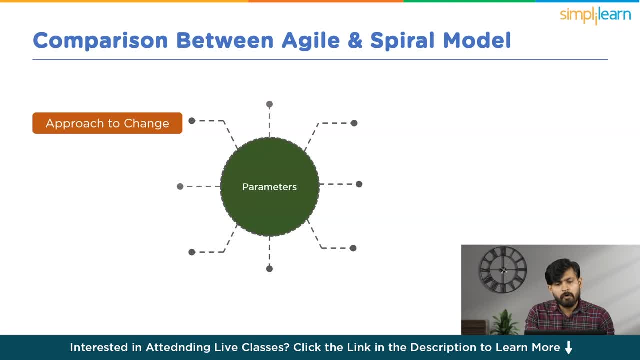 and adaptability. The agile manifests the values responding to change over a following plan, Emphasizing that change is expected and welcomed throughout the development process. Agile methodologies such as scrum embrace change by allowing adjustments to requirements even late in the development cycle. This iterative and incremental approach ensures 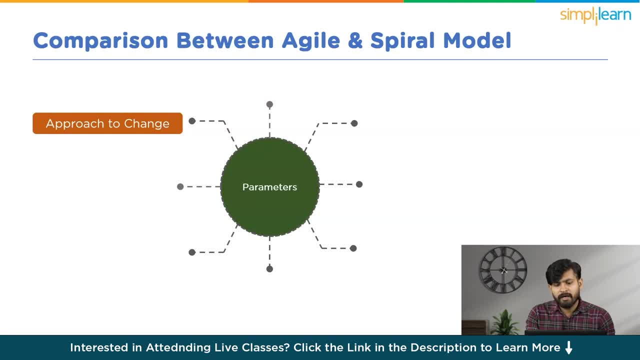 that the product can evolve in response to the evolving market conditions or customer feedback With reference to the same parameter. if I talk about the spiral model, it also accommodates changes, but with a structured approach. The changes can be incorporated in subsequent spirals, taking advantage of their iterative. 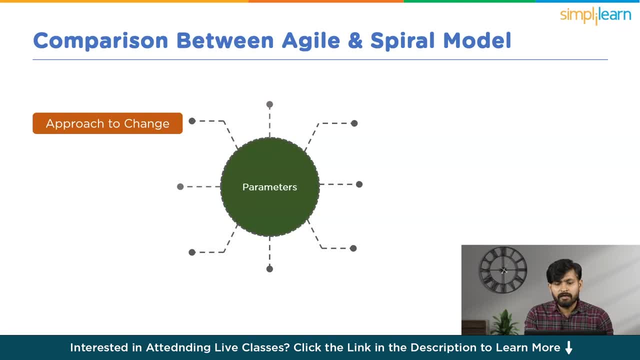 nature of the model. The risk analysis phase in each spiral allows for proactive identification of potential changes, and adjustments can be made based on the insights gained during the iterative cycles. While the spiral model acknowledges the need for change, it does so in the context of risk-driven. 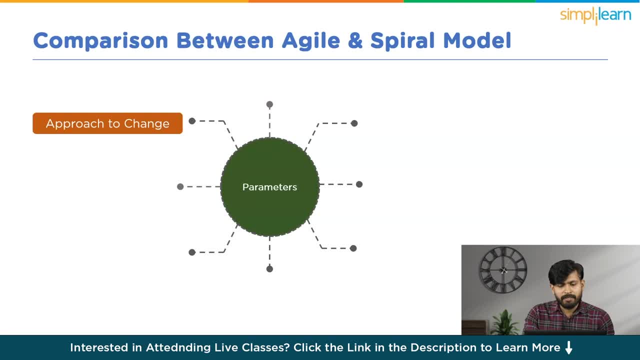 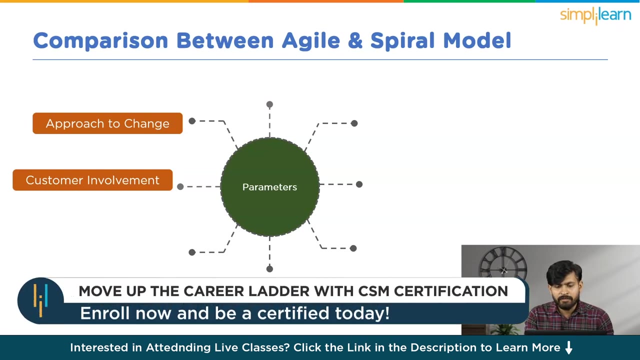 and systematic process. Now let us discuss our second parameter, which is the customer involvement In agile model. it places a significant emphasis on continuous customer involvement throughout the development process. Stakeholders, including customers and end-users, are considered an integral part of the development team. Regular feedback loops, sprint reviews and showcases. 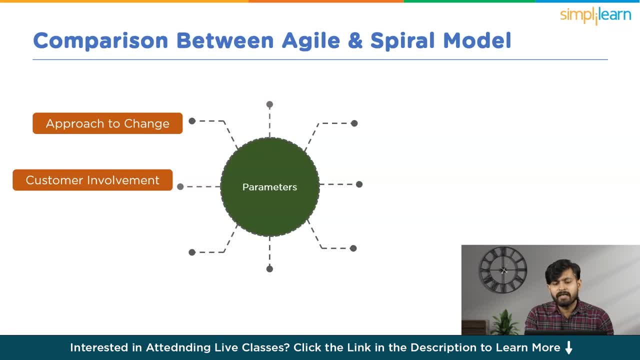 ensure that the customer's expectations are continuously aligned with the evolving product. This high level of engagement contributes to customer satisfaction and helps deliver a product with the desired performance With reference to the same in spiral model. customer's involvement is facilitated through regular reviews and evaluations. Each iteration allows for customer feedback, ensuring that. 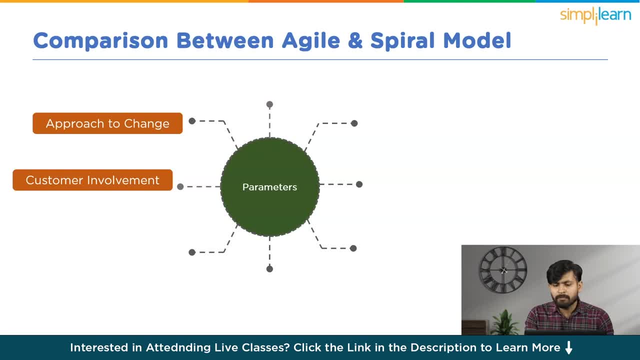 the product aligns with their expectations. While the customer may not be actively involved on a day-to-day basis in agile, the structured approach of the spiral model ensures that customer input is considered and incorporated at various stages of the development. Now let us discuss the third parameter, which is the customer involvement. 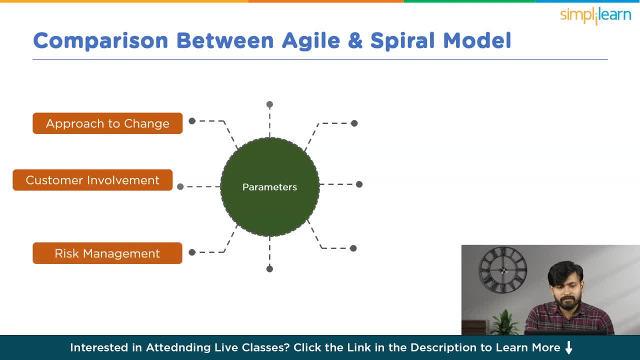 Now let us talk about the third parameter, which is risk management. If I talk about risk management in agile model, it takes a more adaptive and iterative approach to risk management, Rather than having a specific phase dedicated to risk analysis, agile teams continuously assess and respond to risk throughout the development. 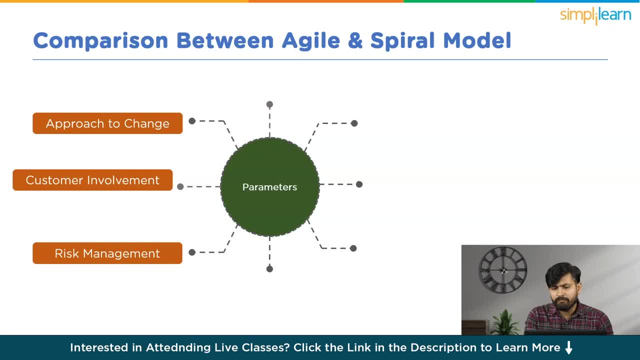 lifecycle. Agile methodologies encourage teams to identify potential risks in early and address them in subsequent iteration, Whereas if I talk about risk management in agile model, it takes a more adaptive and iterative approach to risk management, Rather than having a specific phase dedicated to. 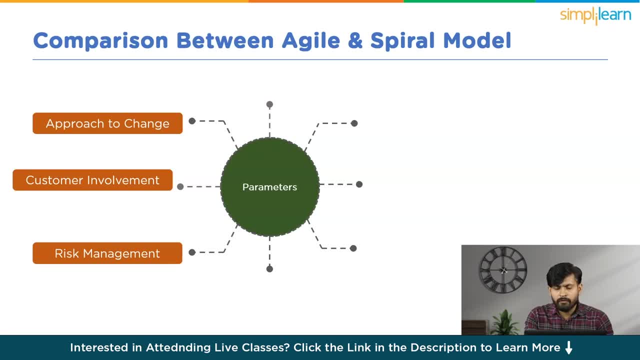 risk analysis. agile teams consistently assess and respond to risk analysis in early and address them in subsequent iteration. Now let us discuss the third parameter, which is the development lifecycle In agile model. the agile model is explicitly designed with a focus on risk management. 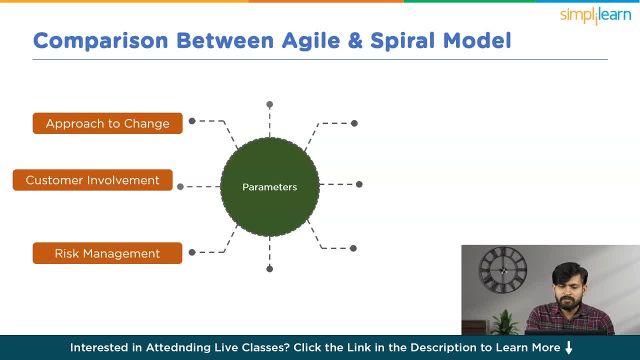 The risk analysis phase, which occurs in each iteration, involves a systematic evaluation of potential risks and the development of strategies to mitigate them. This approach ensures that risks are identified and addressed in a structured manner, contributing to reliability and robustness of the final product. Now let us discuss our next parameter, that is, the development lifecycle, The agile model. 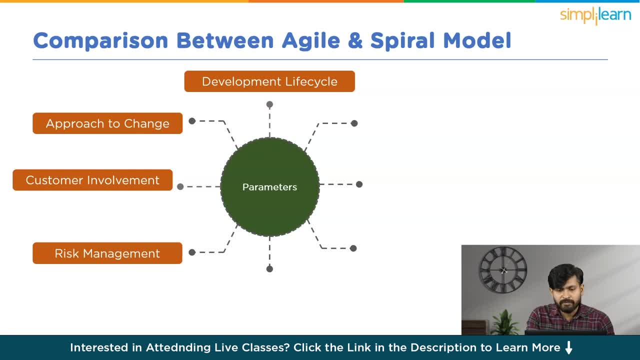 development lifecycle is a very important component of agile development. The agile model development lifecycle is characterized by short time box iterations, or sprints. Each iteration involves planning, execution, testing and delivery of a specific set of features. The development cycle is continuous and iterative, with product evolving incrementally in response. 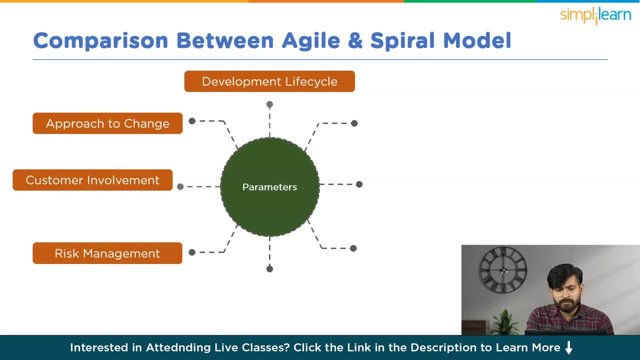 to feedback. This lifecycle is well suited for projects where requirements may change frequently and delivering a minimum viable product is quickly essential, Whereas if I talk about the spiral model guys, the spiral model's development lifecycle is based on multiple iterations or spirals, each encompassing planning risk analysis. 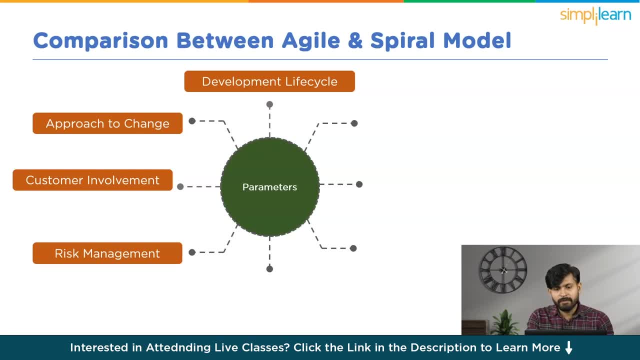 engineering, testing and evaluation phases. The project begins with the identification of objectives and alternatives, followed by the development of a prototype. Subsequent spirals build upon the previous ones, incorporating feedback and addressing risk. This structured and iterative approach is particularly effective for large, complex projects where systematic 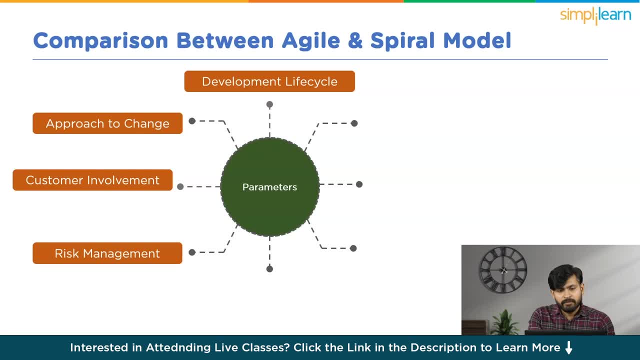 risk analysis is crucial. The project is based on multiple iterations or spirals, each encompassing planning and evaluation phases. Next is suitability for project types. Agile is well suited for projects with dynamic or rapidly changing requirements. It thrives in an environment. 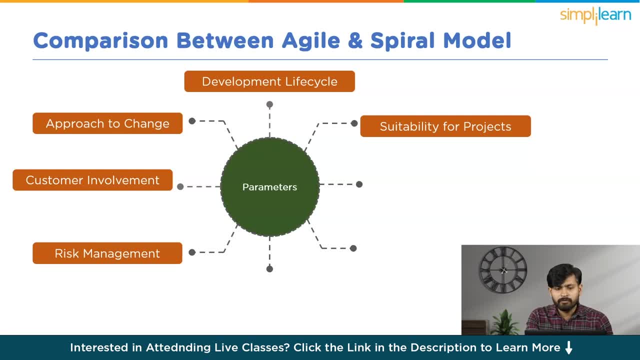 where flexibility, adaptability and quick responses to market changes are essential. Agile is often favored in industries such as software development, where need for innovation and responsiveness is very high, Whereas if I talk about the spiral model, guys, the spiral model is ideal for large. 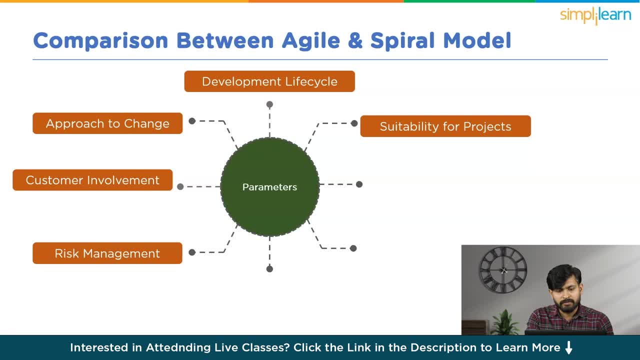 complex projects with uncertainties and evolutions. Next is suitability for project types. Agile is well suited for projects with dynamic or rapidly changing requirements. It thrives in an environment where flexibility, adaptability and evolution are essential. It is often adopted in critical systems such as aerospace. 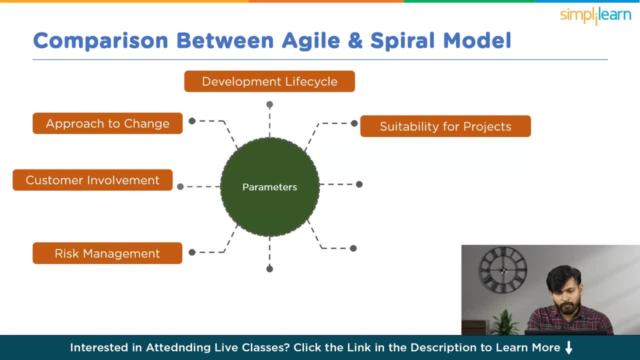 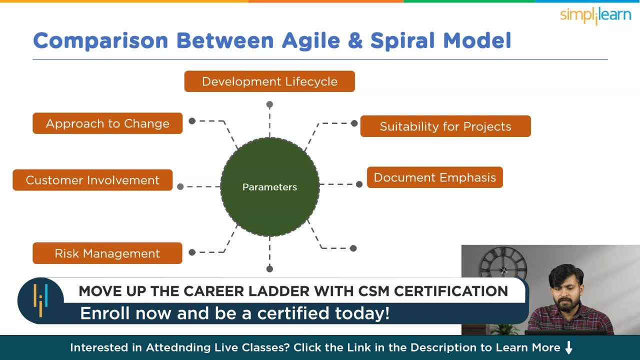 defense and healthcare, where risk management is paramount. Now let us discuss about the document emphasis. Agile prioritizes working software over comprehensive documentation, as stated in the Agile manifesto. While documentation is essential, Agile methodologies emphasize that the primary measure of progress is a functional and valuable product. Agile- 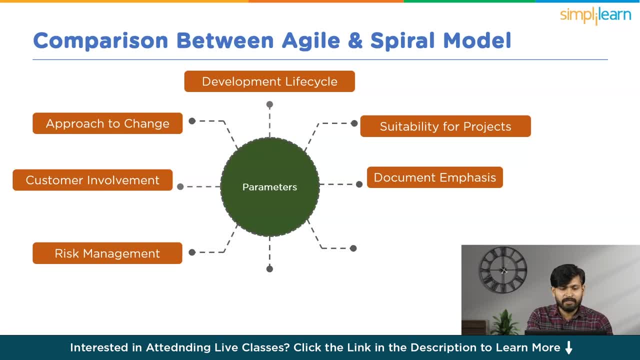 tends to be lightweight and focused on facilitating collaboration and understanding within the team. If I talk about the spiral model guys, the spiral model balances the need for documentation with an emphasis on risk analysis and management. Each iteration involves documentation of objectives, alternatives, risks and strategies. The emphasis on documentation supports a systematic 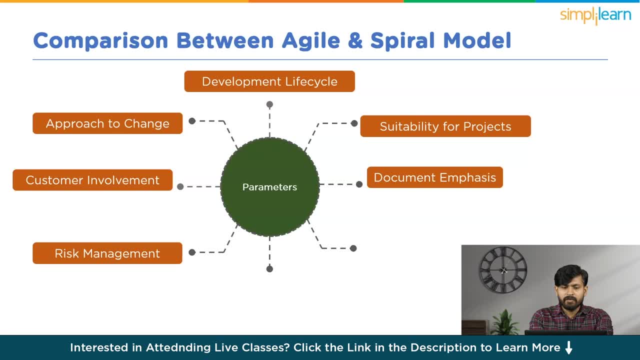 approach to development, providing a comprehensive understanding of project complexities. Now let us discuss the next parameter, that is, iteration or iterative nature. If I discuss the iterative nature of Agile, it is quite inherently iterative, with frequent release and continuous improvement throughout the development life cycle, Whereas in spiral model it embraces iteration refining. 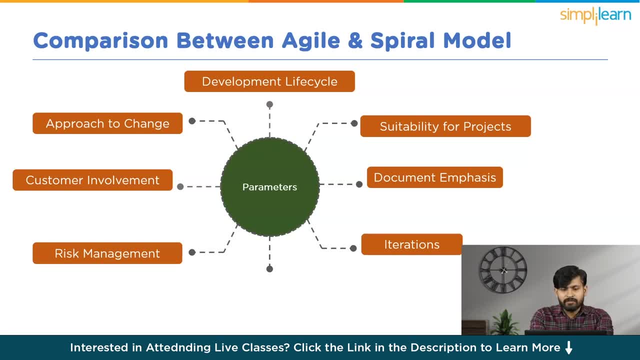 the software through multiple cycles, while managing risk at each phase. This iterative nature allows for ongoing adjustments based on feedback and insights gained during each iteration. This approach is particularly useful for the development of Agile. It is particularly effective in projects where systematic and adaptive developmental process 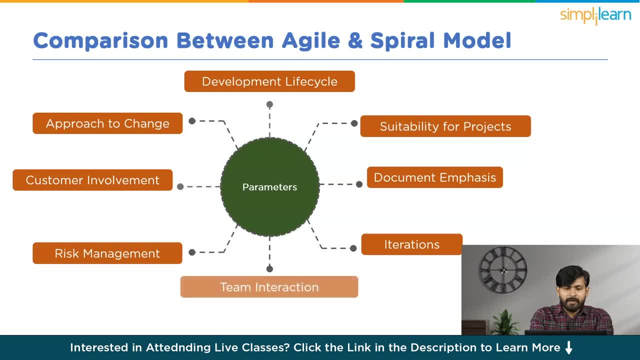 is necessary to address the uncertainties Now. final point, that is, communication and team interaction. If I talk about agile model guys, communication is a cornerstone of agile methodologies, emphasizing the importance of face-to-face interactions within the team, Daily stand-up meetings, sprint planning. 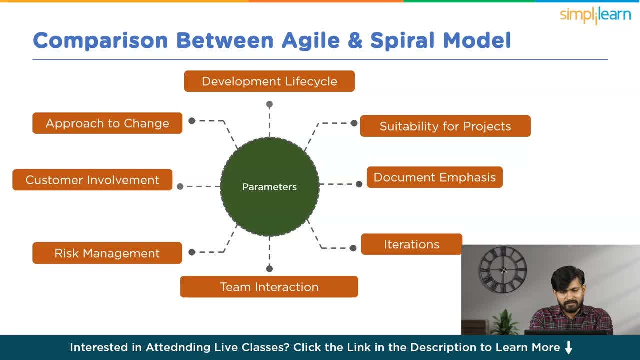 sessions. collaborative discussions are integrals to agile success. This emphasis on communication helps the team members to align on project goals, impediments are quickly addressed and knowledge is shared effectively. This collaborative communication fosters a sense of shared ownership and accountability within the team. 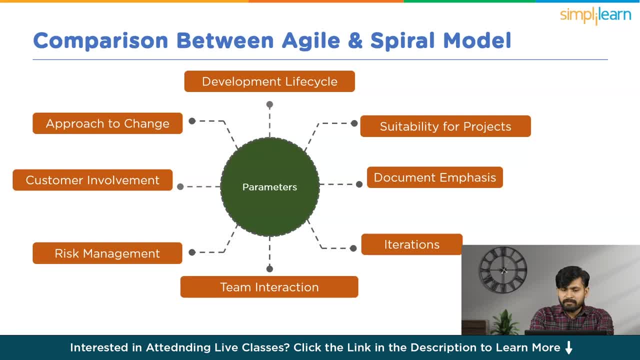 If I talk about spiral model guys, while communication is essential in the spiral model, the formalization of communication process may vary. The model encourages communication between team members, stakeholders, management, especially during the risk analysis phase, and subsequent team iteration. However, the level of formality in communication may depend on the specific